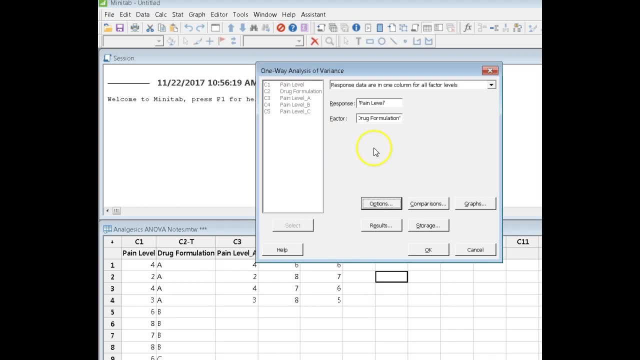 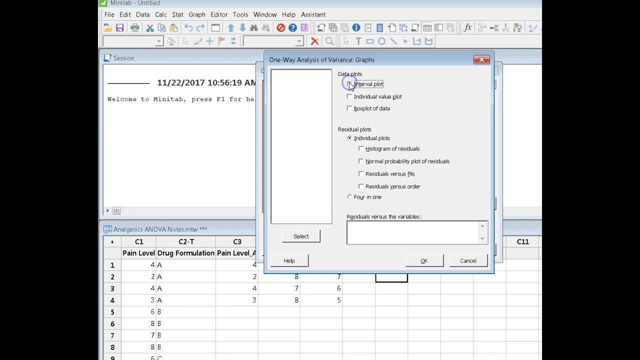 Whenever you run ANOVA, you should always specify graphs. Minitab by default will give you an interval plot. I don't find that very useful. You want to show box plots, because box plots will show us more or less whether our data look like they might be symmetric and normal, And the other thing. 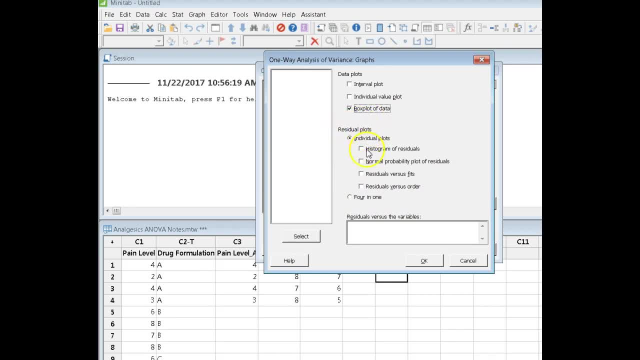 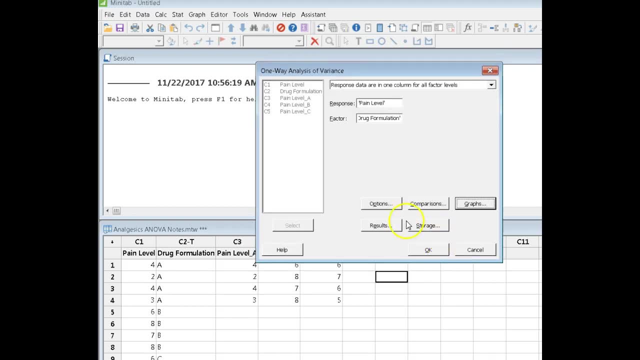 as your notes talk about, is that there's a bunch of assumptions. So if you run a enez and you look at your results here, there's also a bunch of assumptions in here. Just to make sure these are all true. there's a lot of assumptions you want to add, Just like in regression, do a 4 in 1 plot, Say okay to that. There is a. 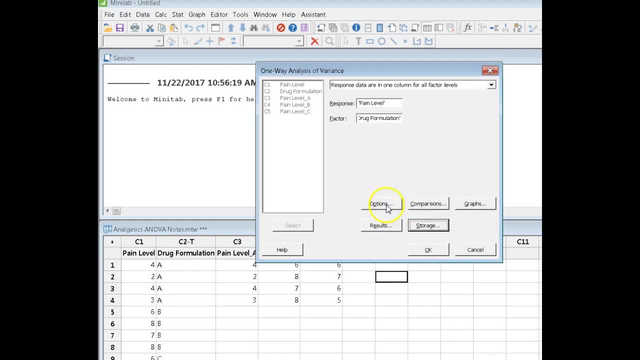 button here that says storage, and just in case you got to check on the normality of your residuals, Just like with regression, you can get Minitab to save them in your spreadsheet. Say okay to that. Alright, now there is a button here for options. 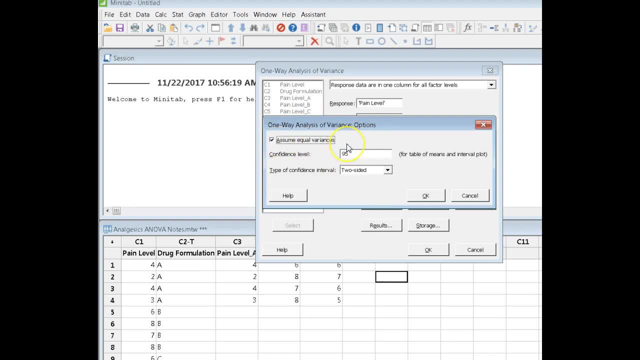 Minitab by default runs and controls the variables. There's a bunch of assumptions. You can get Minitab to do anything you'd like to do, but it's not THAT easy. runs this test with the assumption that the variances are equal and that is the 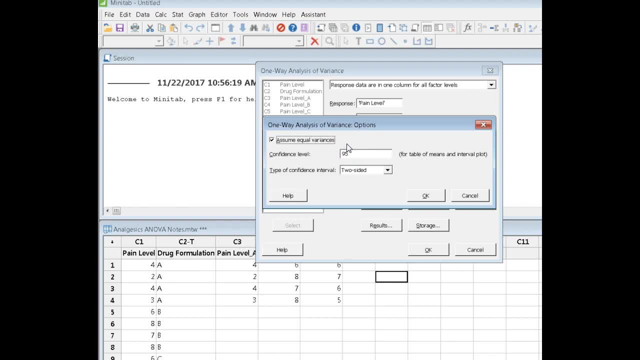 way we are going to run it in this course. so keep that checked on and when it comes time to run the two keys test, you can specify here what level of confidence you want to use, and we want to use a 95% level of confidence. I'm. 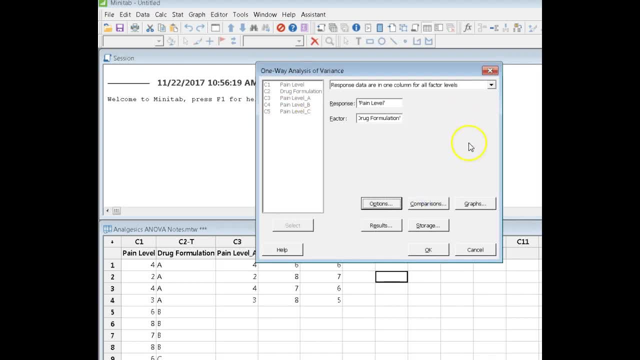 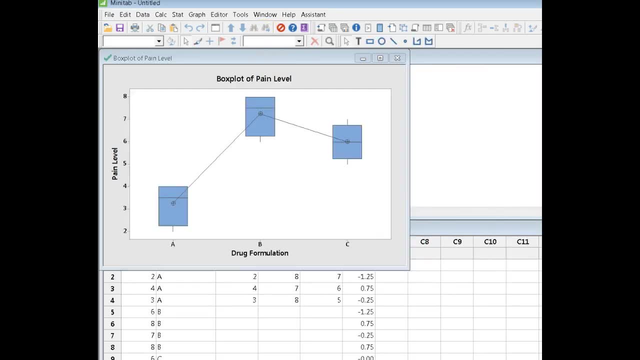 going to leave that alone. say okay to that. all right, at this point I'm going to say okay and I'm going to move that baby out of the way and talk about it in a minute. so before I go, look at my data. as I've already talked about in the last, 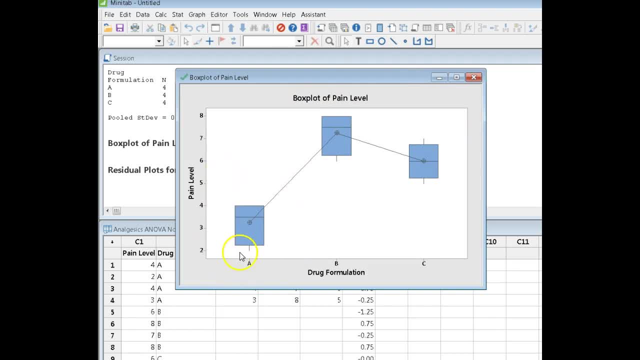 video I can see that drug A gives me generally lower levels of pain than the other two, and there may or may not be a difference between B and C. all right, we want to know whether or not the spread from max to min is roughly the same for. 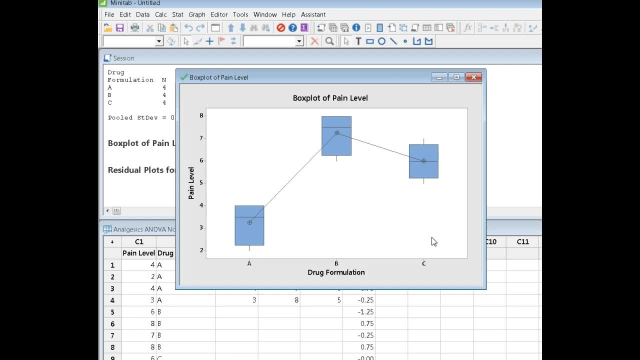 each of the three keys tests groups, and that does look to be the case. I want to see whether my data are normal. that looks pretty symmetric and normal. these two are negatively skewed. we should check these, but, as I said in the previous video, this is of limited use to. 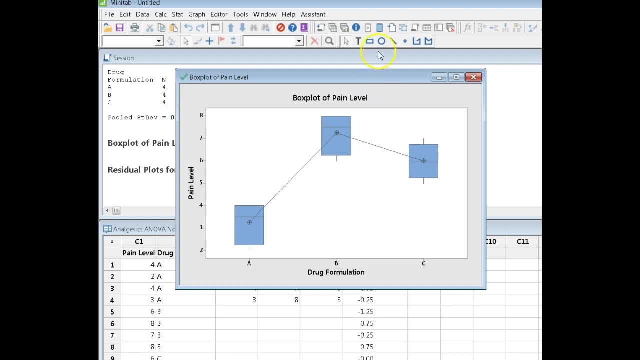 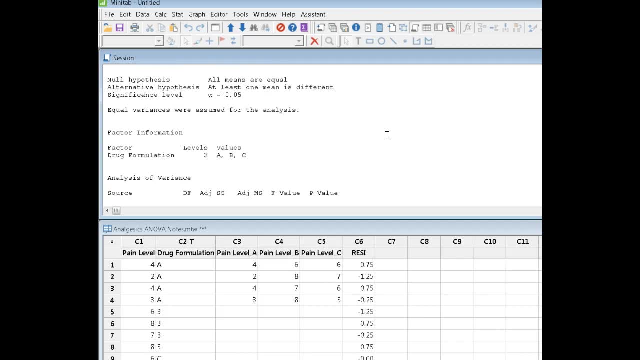 you because you've only got four numbers and how are you really going to prove normality with four numbers? all right, shrinking that down. I would scroll up here and for your assignment and for your final exam, I will expect you to copy and paste all that information and you can go all the way down here to this if you want. all right. 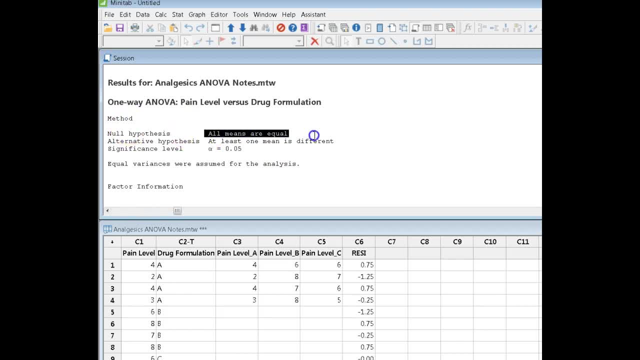 let's scroll up and see what this said. the null hypothesis is: all means are equal versus at least one of them is different, and we told Minitab to do everything at ninety-five percent level of competence, which, of course, is five percent level of significance. tells us it's running the test, assuming equal. 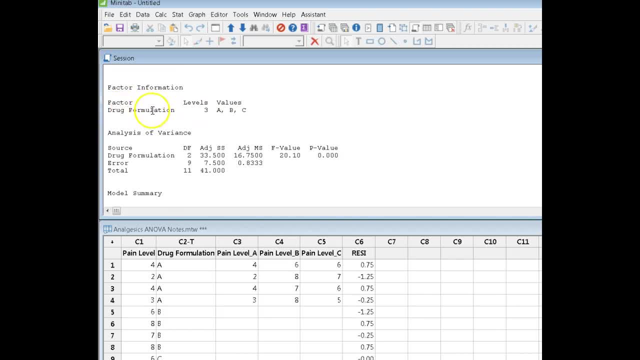 variance. so that's a good way to prove normality. these tests are all the same. there's no difference between them. It gives me my factor information. My factor I call drug formulation. There are three of them and it just tells me what I call them. Okay, then it gives me the. 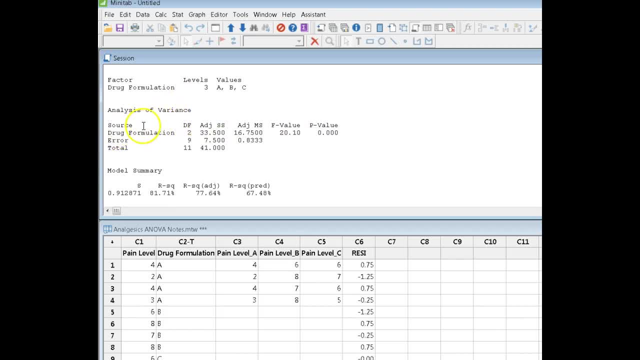 table for the analysis of variance. So you get the source of variability due to your treatment, which is our drug formulation, and due to random error. Minitab calculates the degrees of freedom, the sum squares, the mean squares, gives us our F statistic and the associated p-value. And really, what do? 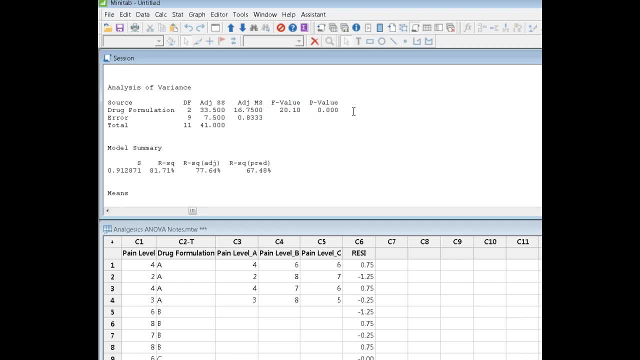 we really want to know out of this. We want to know what's the p-value. All right, so p is 0,, which is smaller than 0.05,, which means we reject that statement and we know at least one of these groups is different. All right. 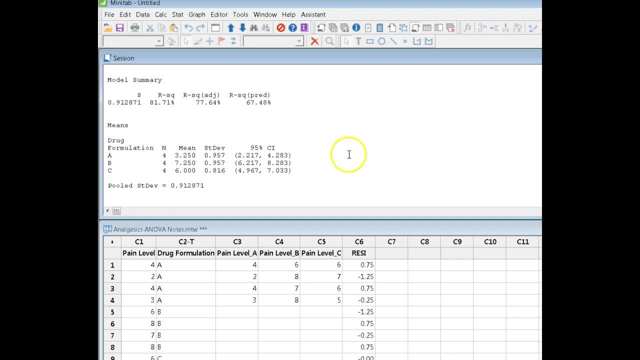 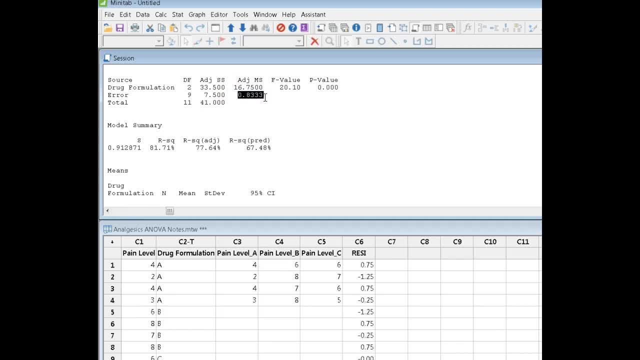 mse. This is the variance within all of your groups and it's calculated by taking every data point and finding out how much it deviates from the group. mean that it's from: If you take this number, which is a variance term, and you take 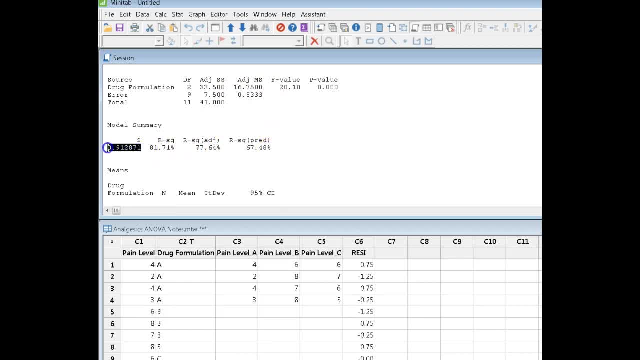 the square root of it, you will get this thing that's sometimes referred to as the residual standard deviation. So what does this number tell me? It tells me that, on average, these points deviate from their group means by roughly 0.913 of a. 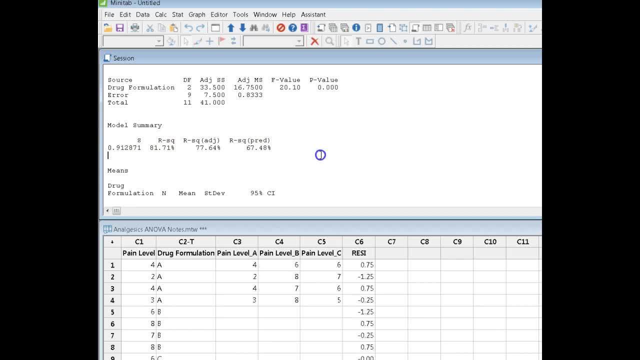 pain level unit. whatever, that is All right, I'm going to ignore the r-squared business And down below here, Minitab is giving us some summary statistics on these groups. And notice, Minitab, I got the s right there at 0.912,. calls it the. 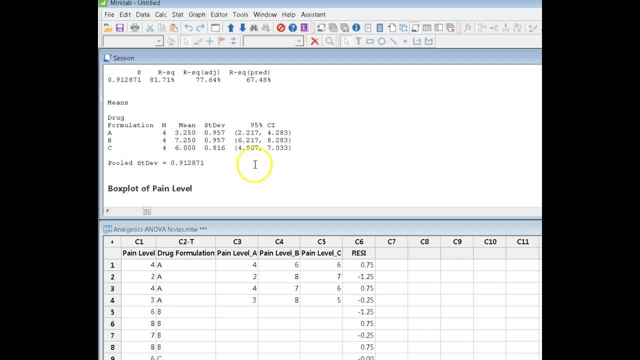 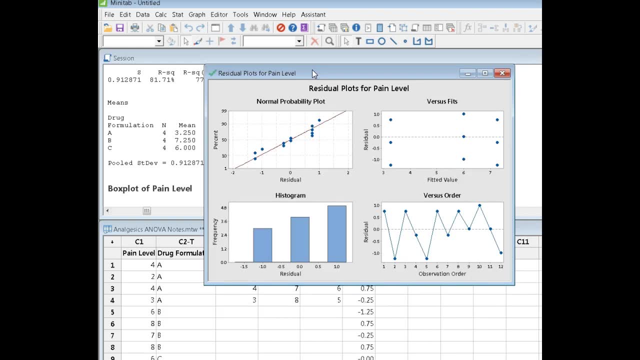 pooled standard deviation, which is what your textbook refers to it as. All right, before I go any further, I want to give you a little bit of information about the residuals. So the assumptions for ANOVA are that your data were randomly and. 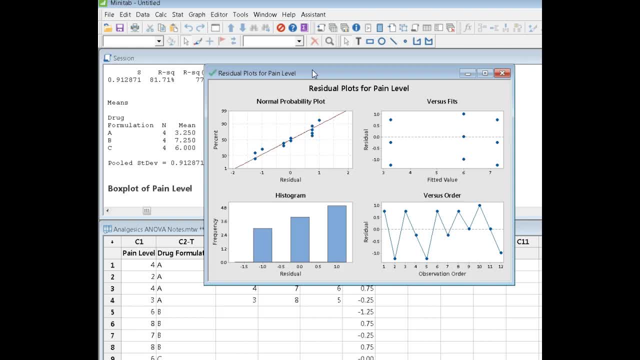 independently picked. Okay, we already talked about this. These people were randomly assigned to the three different treatment groups. As for the independents, well, we may or may not know whether or not that's true. We have to look at the distribution of our data, So each of our box. 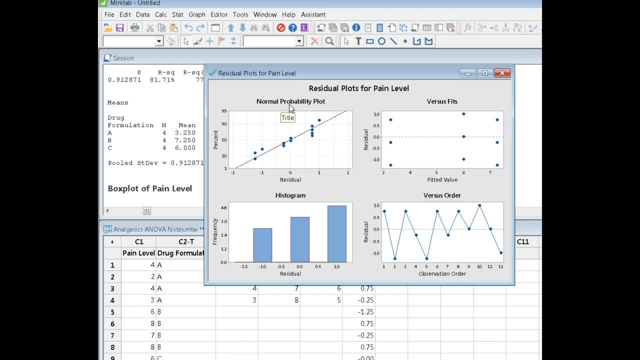 plots look to be reasonably normal, but I will go run a Ryan joiner here. same as this is roughly the same as this. This tells me that my variance for my residuals is equal and I saw that on my box plots- And these are the two plots we want to look at. We're going. 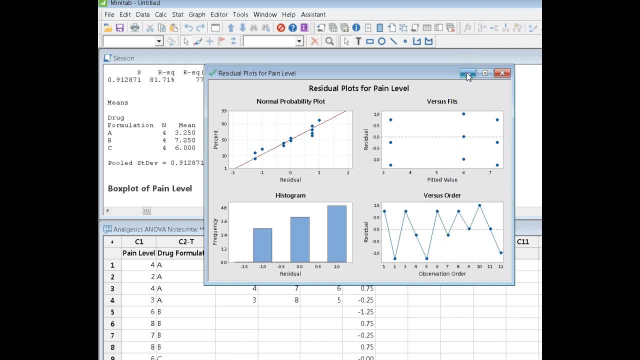 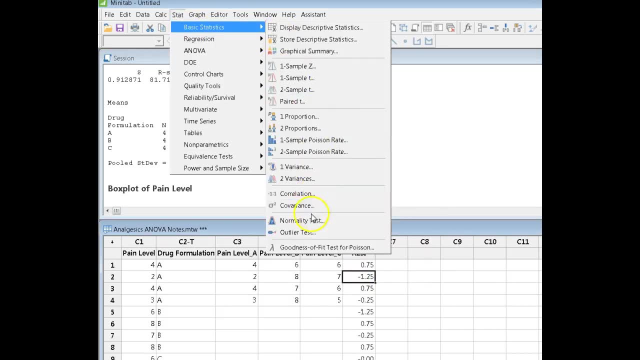 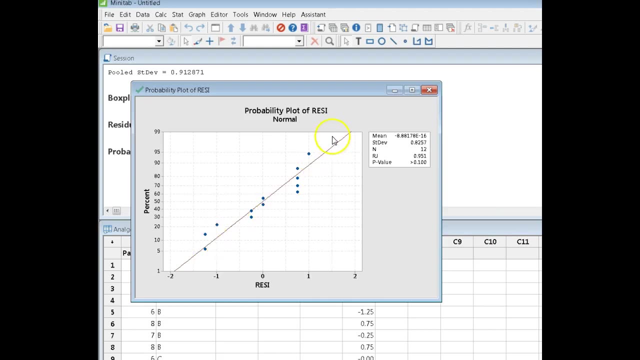 to ignore this one down here, All right now. what else did I want to do before I go any further? I've got my residuals right here so I could go in run a normality test on those residuals and my Ryan Joiner test tells me my residuals are normal because that p-value is greater than 0.1.. 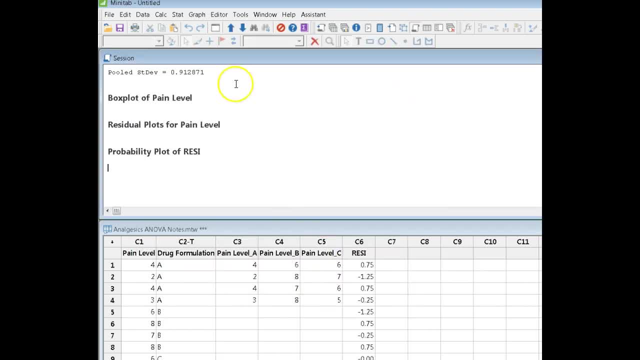 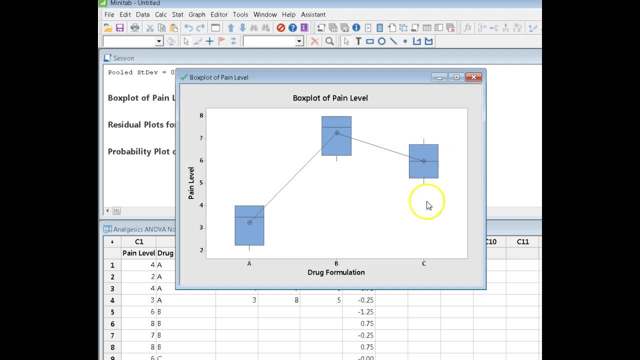 All right, that's fine. The other thing that I wanted to have a look at: hang on now, let me go back: box plots. Okay, this group here looks very normal. a and b. Well, I don't want to. 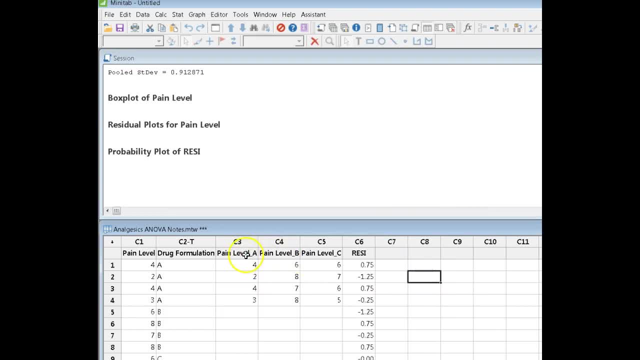 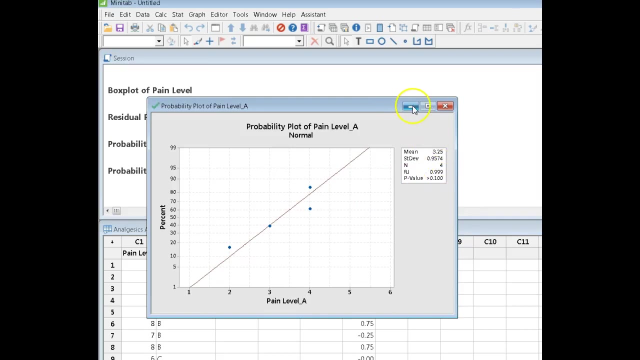 know. Now I've got a and b right here. That is an advantage of having your data in separate groups. So let's go determine, for what it's worth, whether group a is normal and it says p greater than 0.1,. 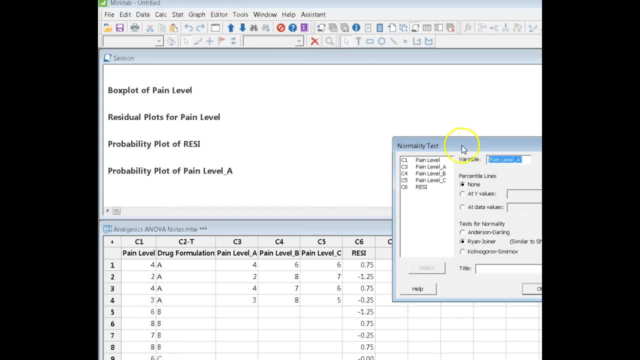 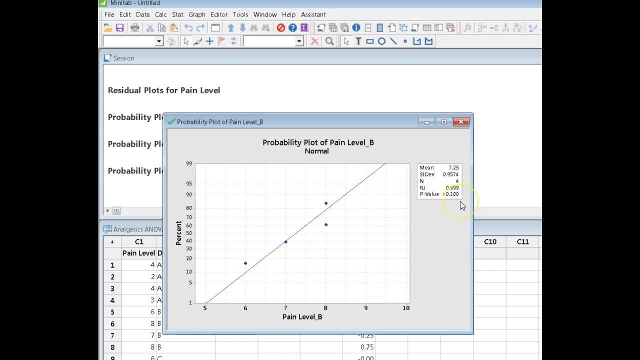 so they're normal. And if I do that again this time for group b, and we're also told they're normal with a p-value greater than 0.1. And again, for what that's worth, because we've only got four data points. 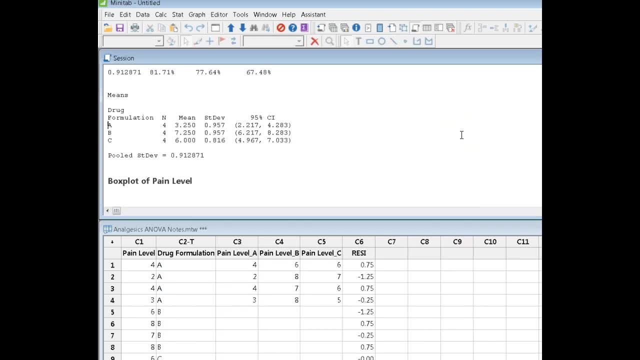 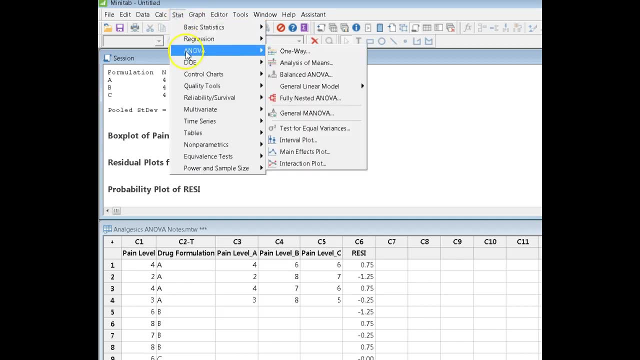 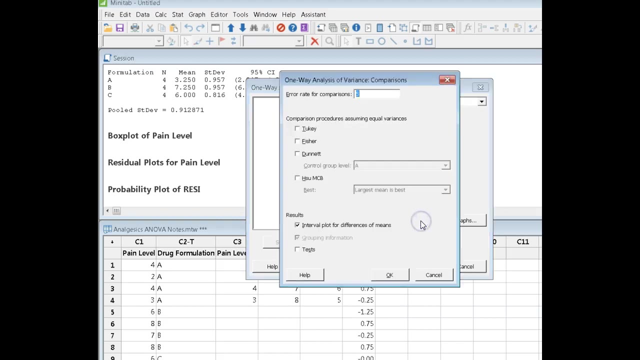 All right, looks like all of our assumptions are met. so that's good. And we know that there is a significant difference in the groups. So now that we know there's a significant difference, we go back to our renova and we hit this button called comparisons, And it's here where you specify what. 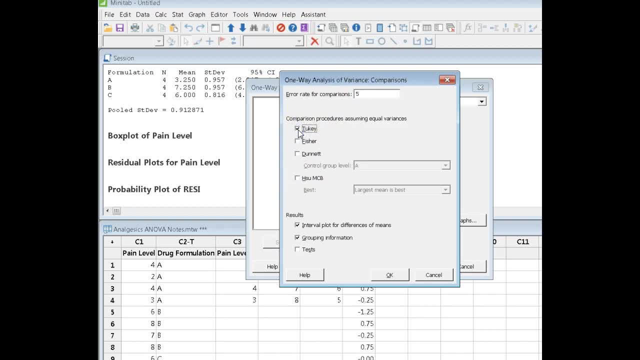 test you're going to use In this course. we're only going to use the test, that we're going to use The two keys And it says: this is a test that's done assuming equal variance. And we already know now that we do have equal variance. All right, leave all that stuff turned on, say okay and 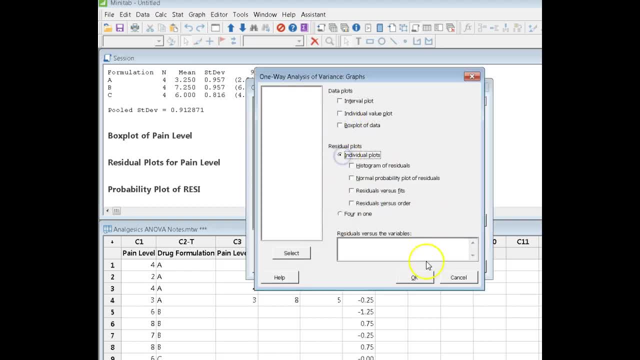 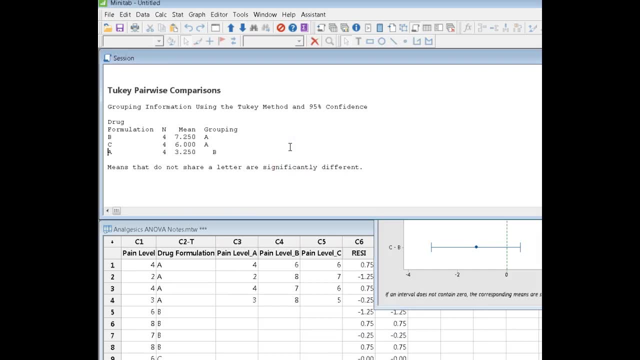 because I've already seen them. I'm going to go turn off these plots right here. Okay, so Minitab gives me. first of all, if I scroll back here, here's what I get out of my two keys, And again: 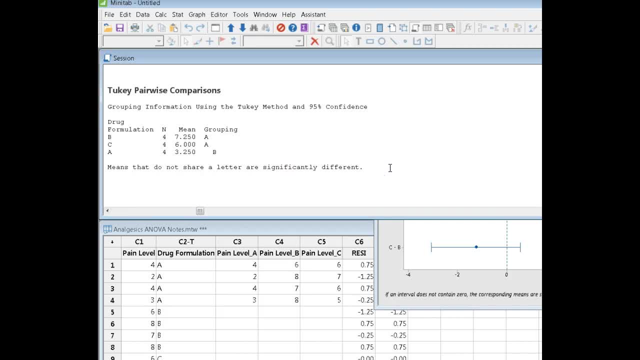 on an assignment or on a final exam. I expect to see this information Because my grouping letters here are both A's. this tells me that these two groups are not significantly different. So that tells me drug formulations B and C are not significantly different from each other. However, they are significantly different from: 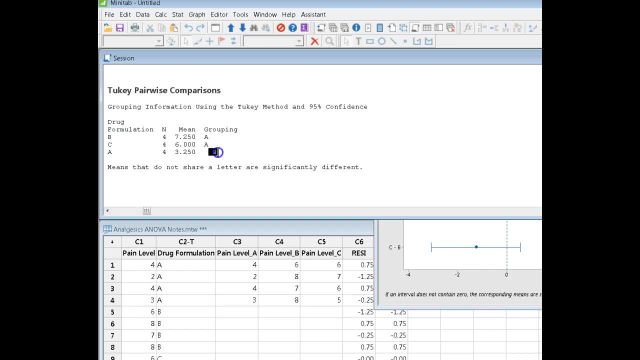 this group right here, because this group has a letter, code B, which is not shared by these two up here. And Minitab always lists these in order of decreasing size of your mean, So it goes from biggest mean down to smallest. In our case, which drug is better? It's the drug that gives the less pain level, which then 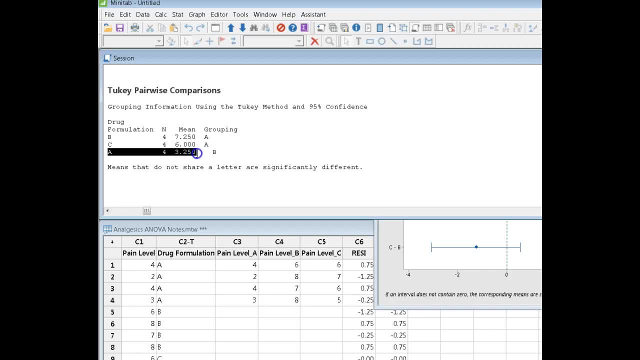 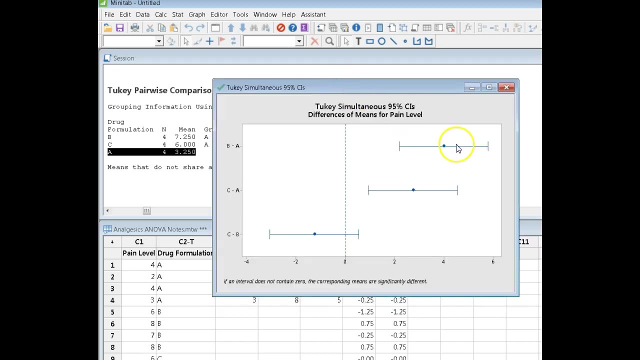 means that drug formulation A is best because it gave a significantly lower average pain level than drugs B or C, and there's no difference between them. And, as I already explained in your notes as well, these intervals help you interpret what is wrong with this. 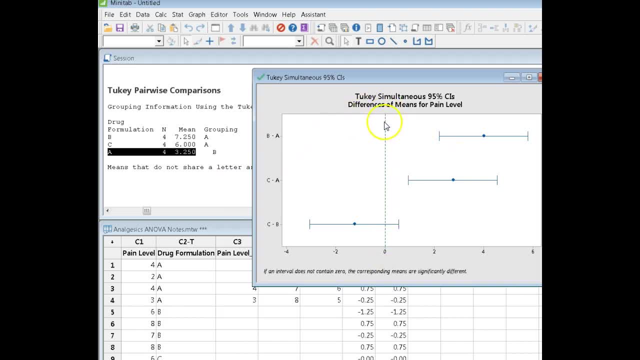 grouping information Intervals. they go through zero, as this one does tells me there is no difference between the groups being compared, so no significant difference between C and B. These two intervals contain all positive numbers, which means in this casegives me higher level of pain than average. So it's about the same as the reports. you can also see evidence for that. There's enough is two up to three. but it means rhyme nosso didi pessoa deum other. So I wanted to let you know that świat emphasized in uppercase the потому jeger. ED 1507, flowią harmony. nãoAKE nahiע uploaded a vertebra de número. bem da gaieta. It was no significant difference between theочь group and the group. not having bled isn't the same meaning here either. These two intervals contain all positive numbers. 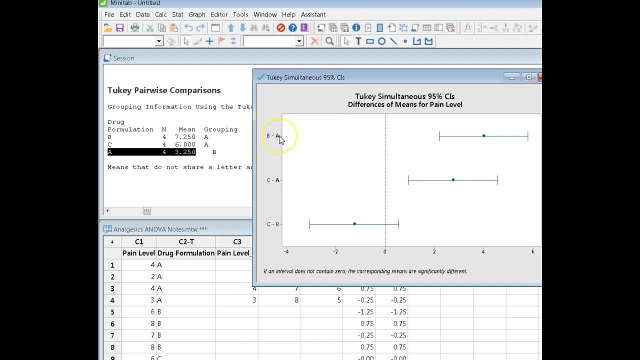 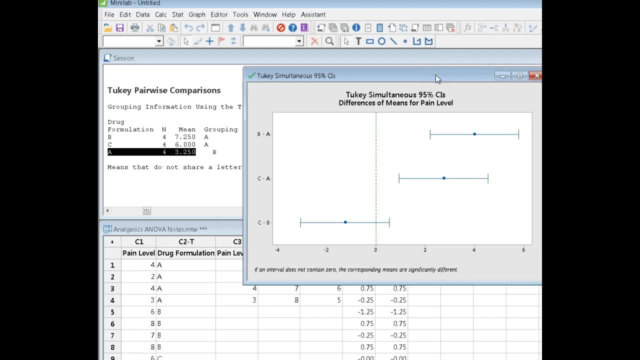 means in this case, B gives me higher level of pain than A and C gives me higher level of pain than A, which must mean that pain formulation, or whatever it is that the drug, a formulation is better at relieving your pain than the other two. now I think that's pretty well it? oh, I was going to show you the ANOVA. 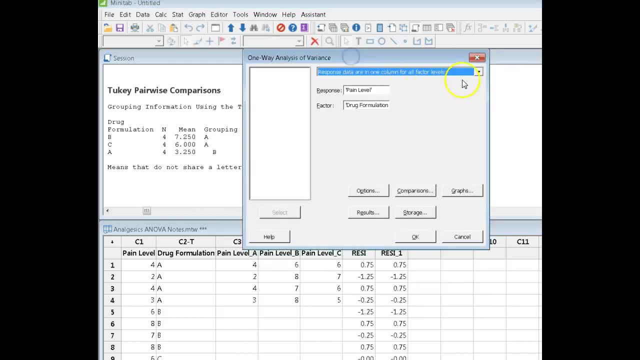 if we run it where our data are all in separate columns. so if that's the case, make sure your cursors down in this box. my data now are in columns 3, 4 & 5. you pick those three and everything else is going to be the same, except when you go. 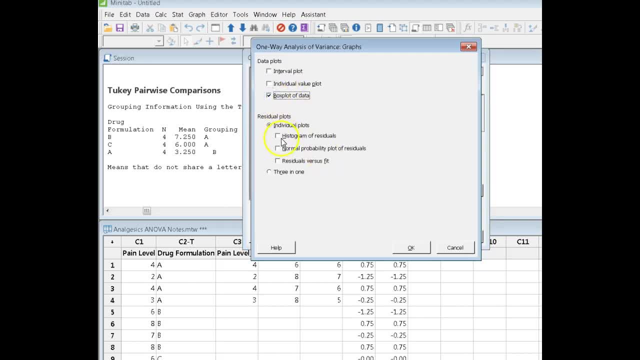 to graphs. you can get box plots, but there is no 4 in 1 plot. you only get a 4 in 1 plot. you only get a 4 in 1 plot. you only get a 4 in 1 plot if the data are all in one column. so Minitab will give me a 3 in 1 plot and 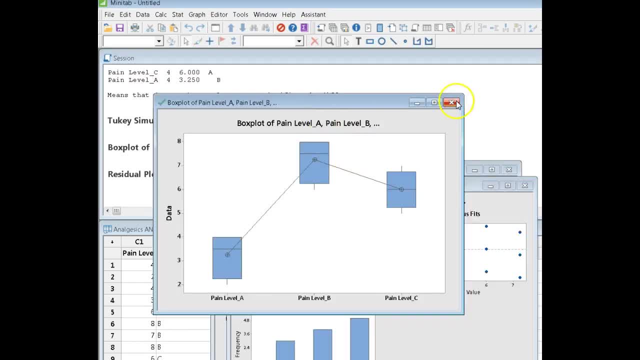 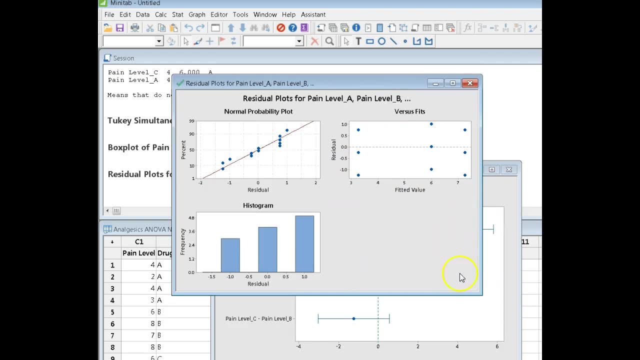 other than that everything else is the same. so I get my box plots. okay, yep, get rid of that. and here it doesn't give me that residuals versus order plot, and the reason is is because when they're all in separate columns it doesn't know what.